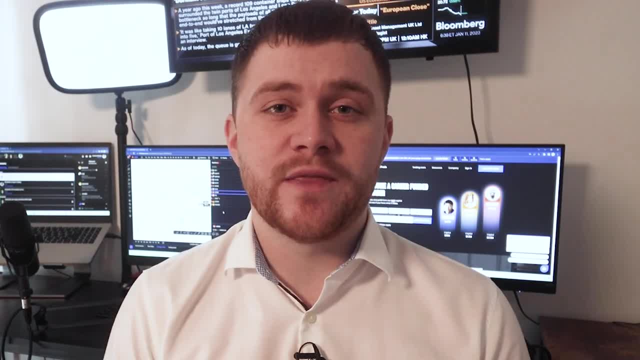 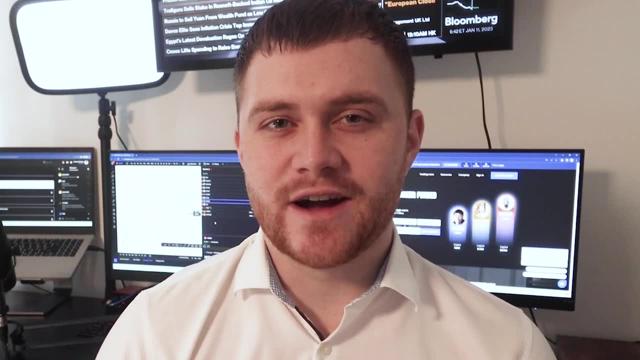 are a representation of money being stripped from the economy and thus a weakening outlook. Okay, so how is CPI calculated? Now, when we talk about how these CPI figures are actually calculated, it can get complicated, but let me break it down simply for you. The calculation: 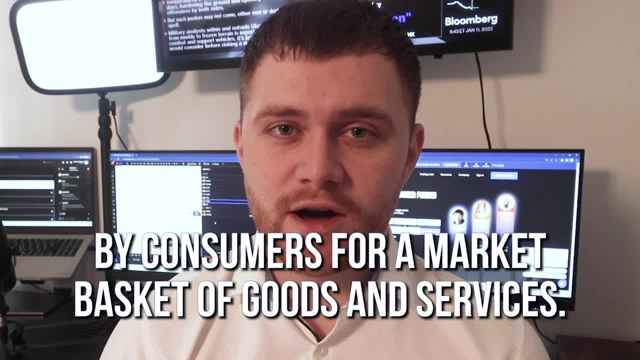 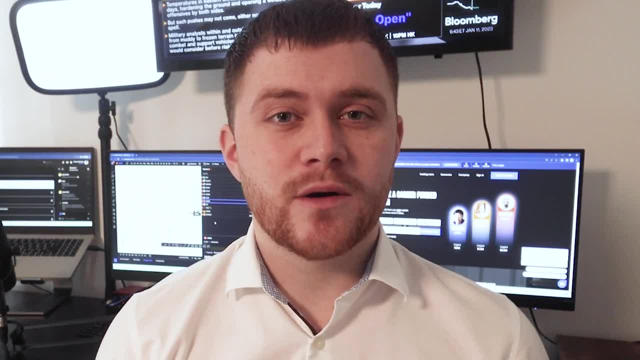 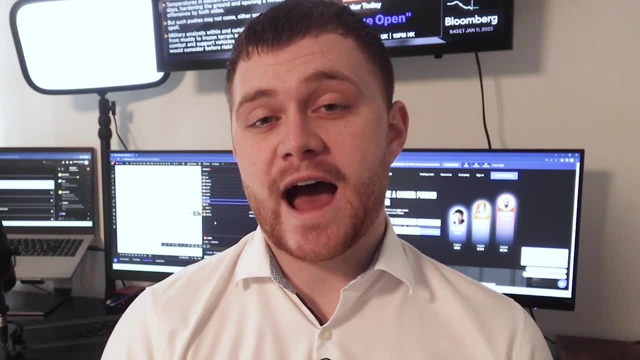 involves taking a measurement of the average change over time in the prices paid by consumers for a market basket of goods and services. And you may think: well, what is a basket of goods and services? Well, essentially we are talking about a theoretical group of products that average 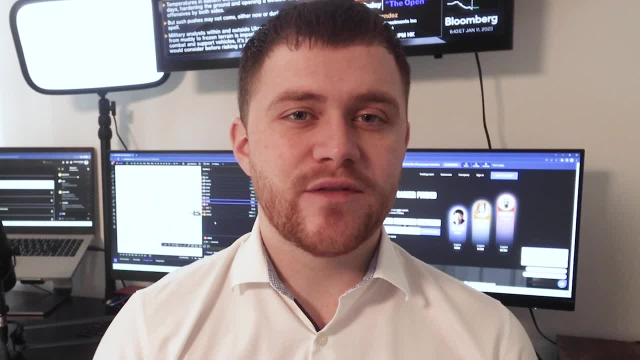 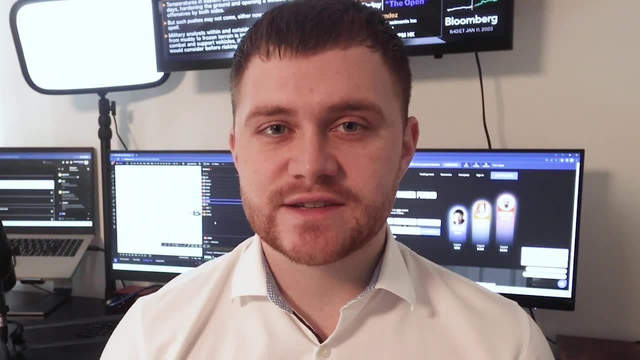 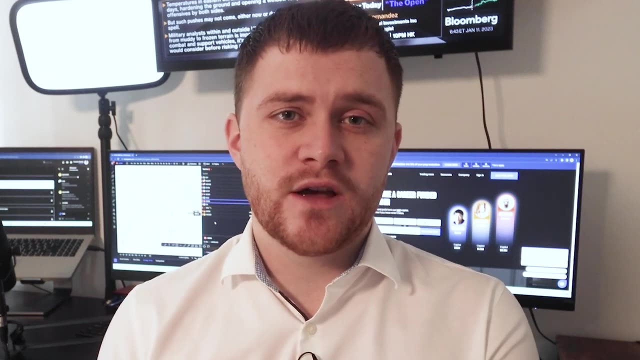 consumers in a country will typically buy, including things such as bread and milk, or housing costs like rents, transportation, education services, medical care and so on, If the price of that basket is higher from one month to the next or from one year to the next. 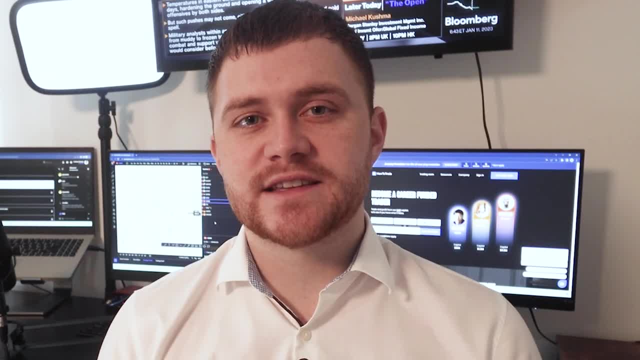 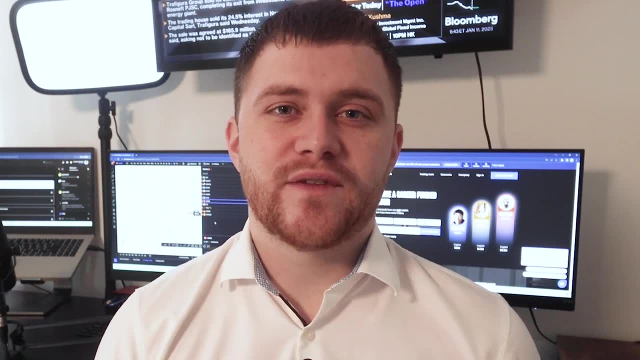 that means prices are inflated and this is the key data for central banks, who in many cases, target 2% inflation. At the time of recording this video, inflation is usually 2% higher. in the US is over 7%, over three times the target. Therefore, it's been the dominating. 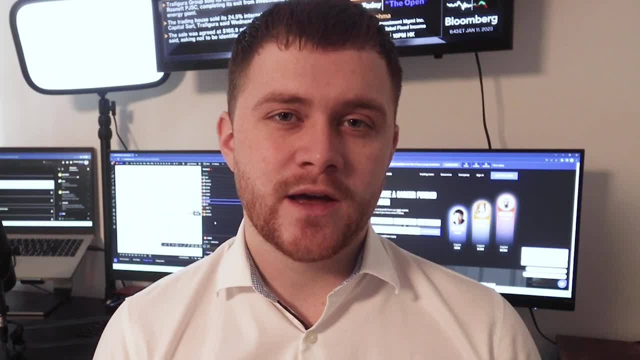 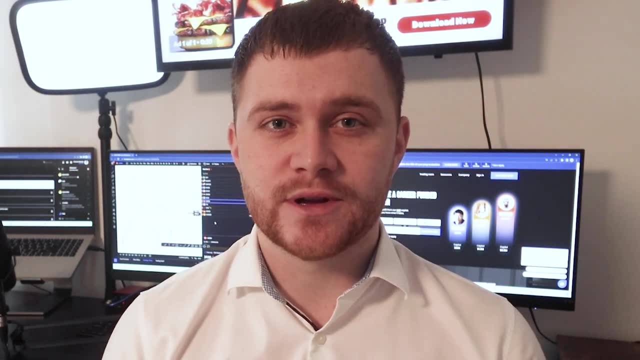 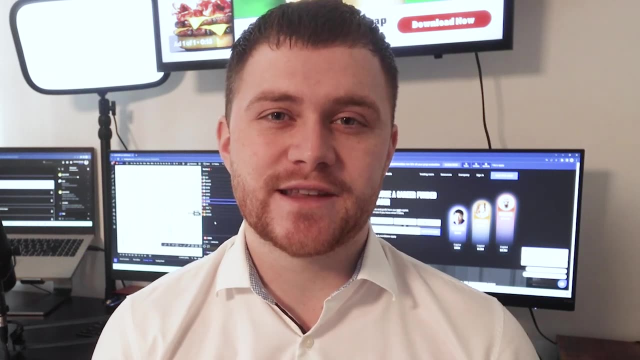 story over the last year and will always be topical. Monthly CPI releases typically cause significant volatility in the markets and they should not be ignored. Let's tune in to our expert analysis in the States, Shane Veneer, to explore the sorts of reactions we can expect to witness. 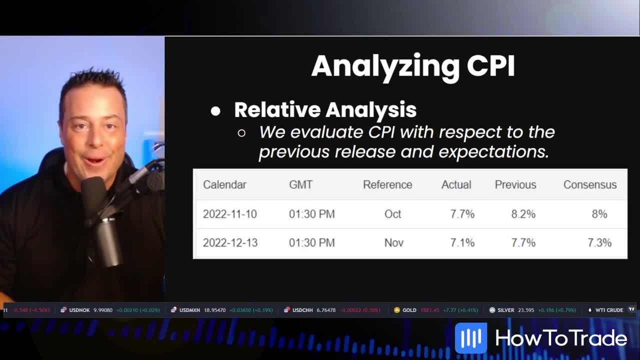 as traders. Thank you, Connor. Now that we know what CPI is, we can talk a little bit about how to analyze CPI in the live market. To do so, we use a device called relative analysis. Now what relative analysis is is we evaluate a factor with respect to its previous release. 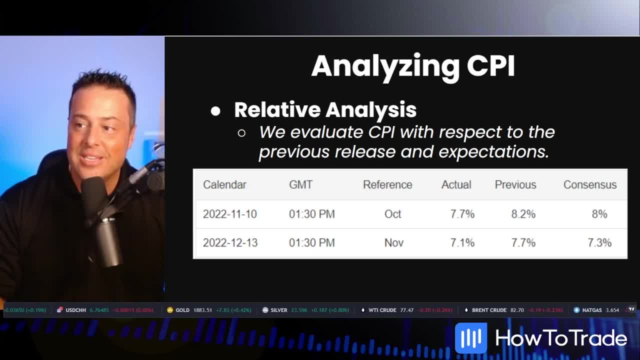 and expectations In the case of CPI. we evaluate CPI with respect to its previous release and market expectations. As an example, you can see back in December. on the 13th of December we had the release of November CPI value. the actual number came in at 7.1% Now that was well below the previous release. 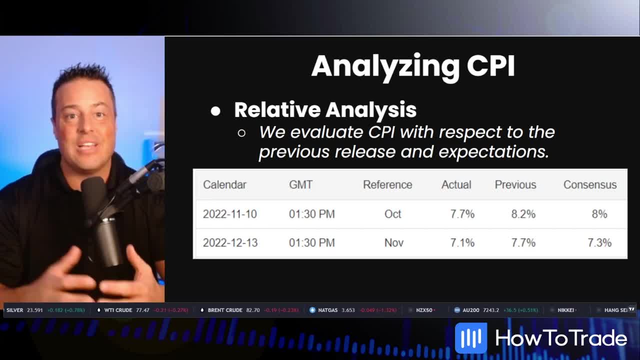 which was 7.7% and consensus expectations of 7.3%. So in this case we can definitively say that inflation did come down, CPI did pull back and that was going to have an impact on the markets, as well as the US dollar commodities, really across the board. So when we analyze CPI, 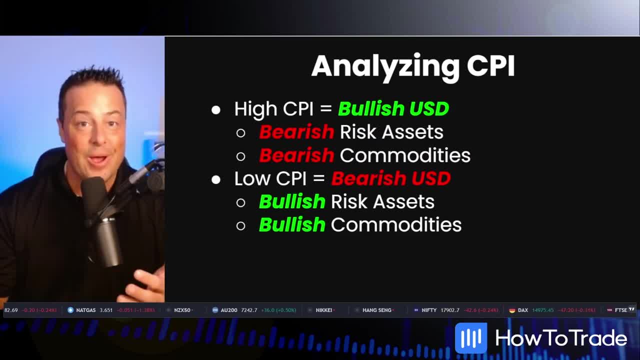 with our relative analysis. there's a couple of different ways that the number can go and a few different impacts that it can have. So let's go ahead and take a look at the number Now. a high CPI reading, which would be one that comes in well above expectations, and 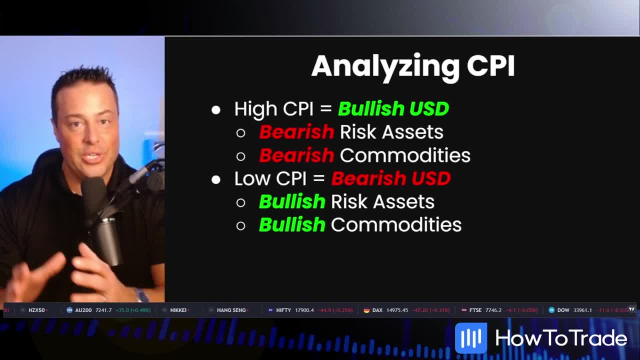 well above the previous release is going to lead to a bullish USD. Now why would that be the case? When we have runaway inflation, central banks get involved. they raise interest rates, they try to reduce that money supply and in doing so they put pressure on things. 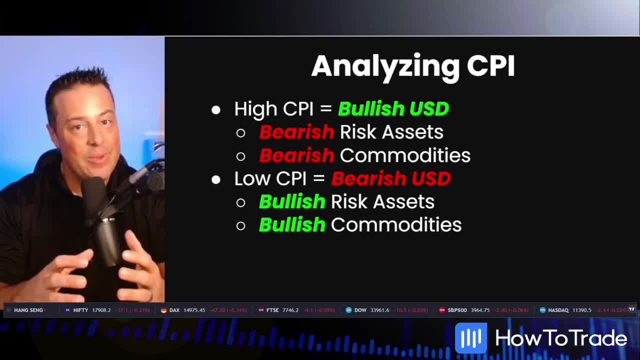 like risk assets and commodities. So a high CPI is a bullish US dollar. That leads to bearish risk asset pricing and bearish commodity pricing. Now, on the other hand, a low CPI, as we just went over, when you have something that comes. 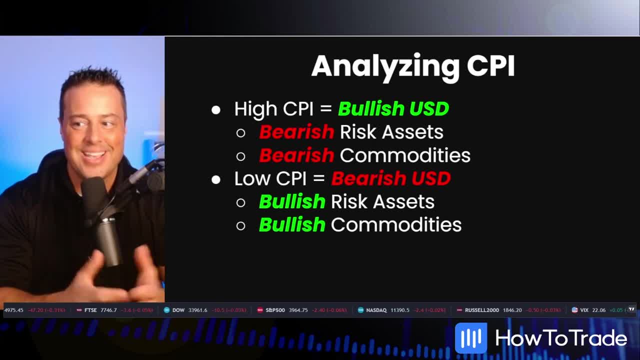 in. beneath expectations and beneath the previous release, it actually leads to a bearish USD. Why is that? Because the central bankers are less likely to step in and intervene to control that runaway inflation. So what do you have? You have a weakened US dollar, which leads 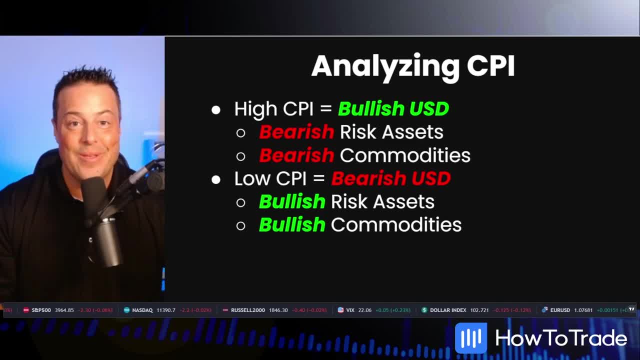 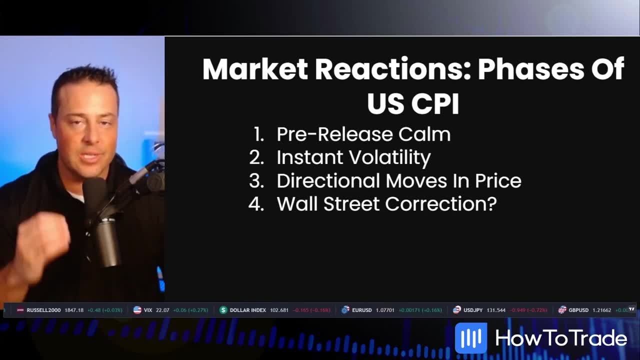 to bullish risk asset pricing and bullish commodity pricing. Okay, now that we know what CPI is and how to analyze it in the live market, let's talk about what we can expect when the number actually is released to the public. In my estimation, there are four distinct phases to a CPI release, and here they are. 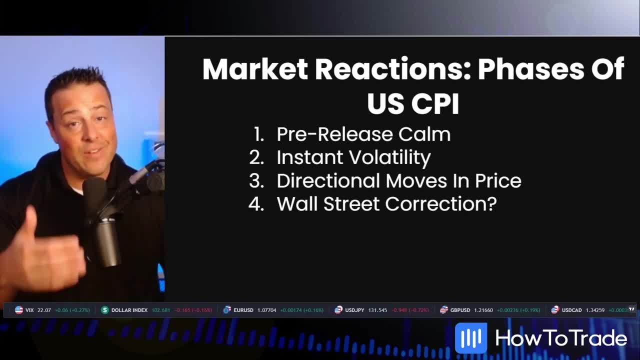 Number one is your pre-market calm. That's when everybody is really waiting for the number to come out. A lot of uncertainty. No one wants to commit one side or the other to the market. Very calm, tight market conditions. Number two: instant volatility. When the number actually is released to the public, a rush. 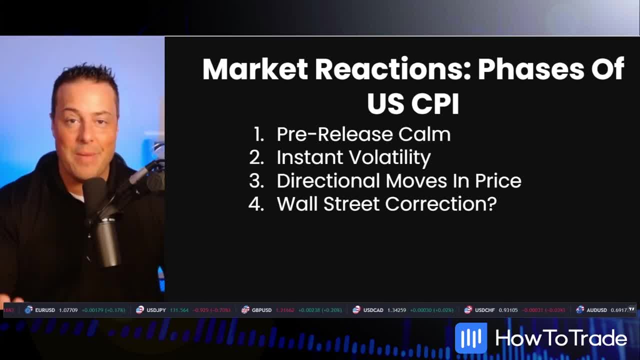 of orders hits the market. Everybody, from institutional traders to momentum algorithms, get involved in pricing. the CPI release Number three. it creates a directional move in price. Now it may be for a very short period of time. We may only be talking about 15,, 20,, 30 seconds, a minute, two minutes. 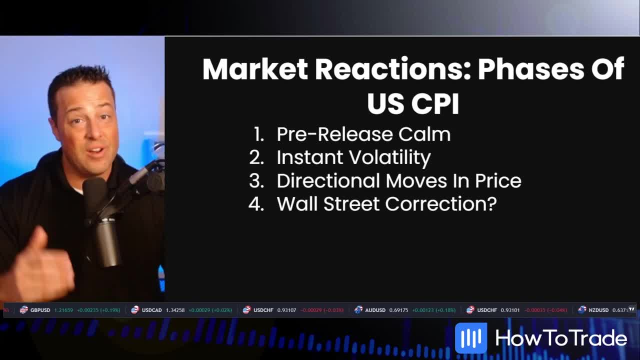 30 minutes. It may be for a short period of time, but typically there's a definitive bullish or bearish initial reaction to the CPI release And lastly, a Wall Street correction. In some cases you see Wall Street on that cash open. 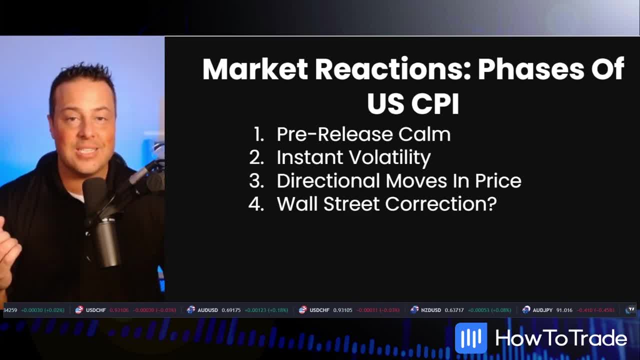 about an hour after a CPI release, You'll see a correction of the price action. You'll see price come off of a bullish move or up from a bearish move. Now it's not an according to Hoyle rule and it also depends on the asset class you're 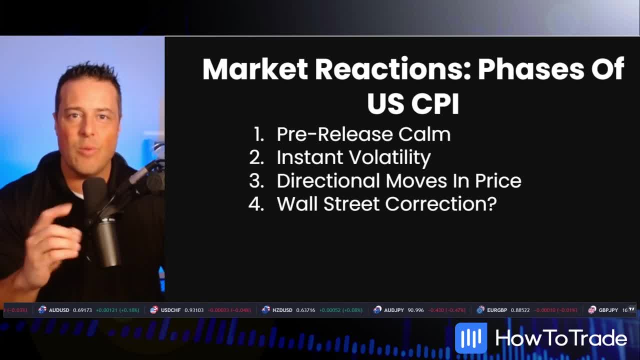 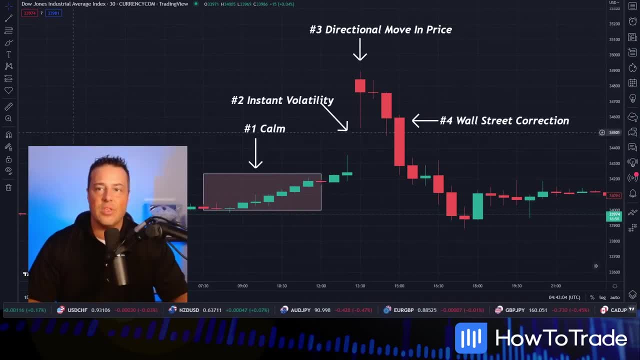 trading. but a lot of times that cash open, that Wall Street open an hour later can produce very different price action than what we saw during CPI. So let's take a look at the pricing charts. This is an example of the US 30 back on the. 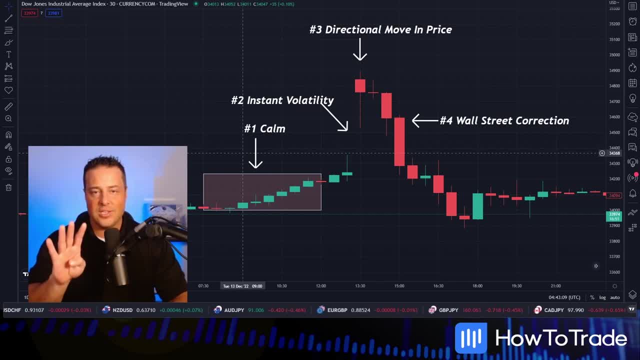 December 13th release of CPI. You can see our four phases are clearly defined. Number one is our calm, very quiet markets, very tight, tight trading conditions leading into the release And then boom, market drop or, excuse me, the. 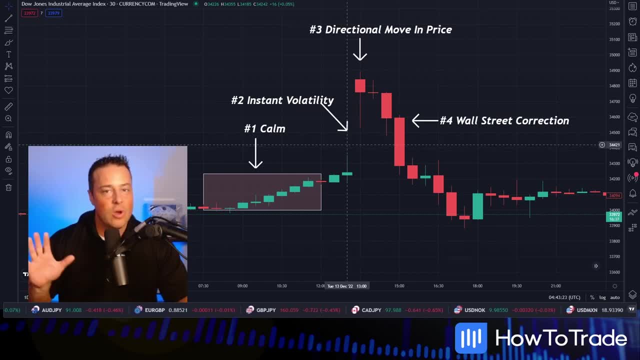 number drops, The market takes off, absolutely takes off. A rush of orders hit. There's no one on the sell side And what does that create? Our number three phase: a directional move in price. In this case, you had an initial directional move to the bull Upwards trajectory of price. 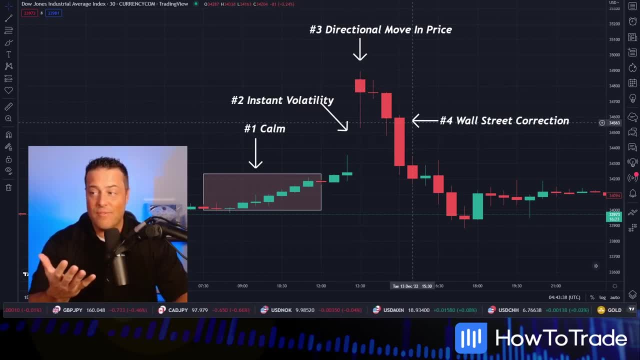 action. And then what happens from our top Number four, our Wall Street correction. As the CPI number becomes priced in the live market, we see a contrary price action to that initial CPI move. Four phases calm before the storm, Instant volatility. that rush of orders creates a directional move in price And in this case, 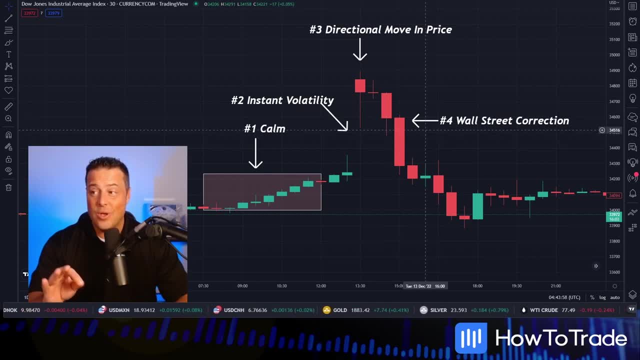 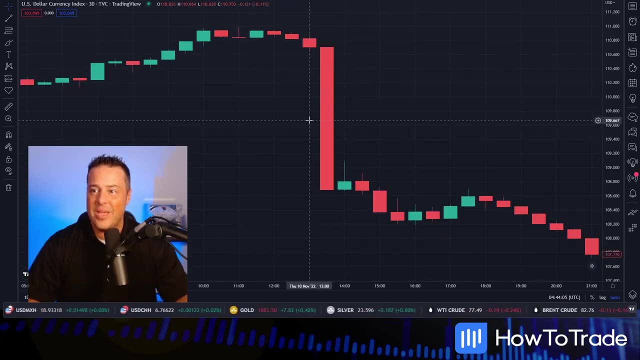 for the US 30. back on December 13th 2022, Wall Street stepped in and corrected the initial reading of the CPI. So fascinating. look at price action and the four phases. It really does depend on which asset class you're trading. This is the November release Now. very similar number, very different. 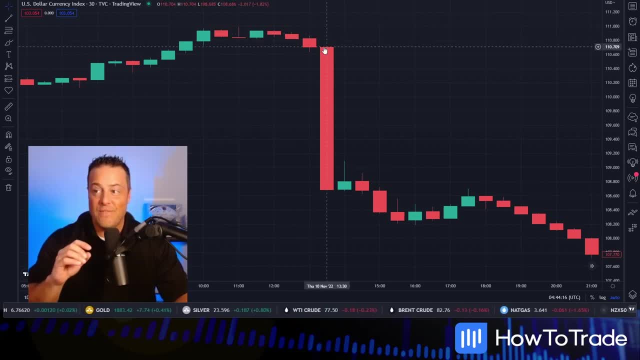 price action. here You'll see: phase one: calm before the storm. Phase two: number comes out. rush, an absolute rush of orders hits the market. If you're a stock market, you're going to get a crash. If you're a stock market, you're going to get a crash. If you're a stock. 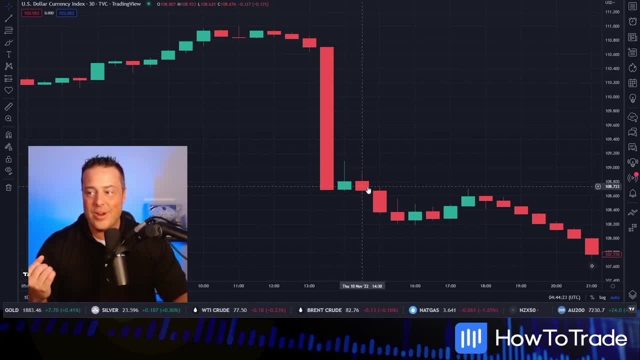 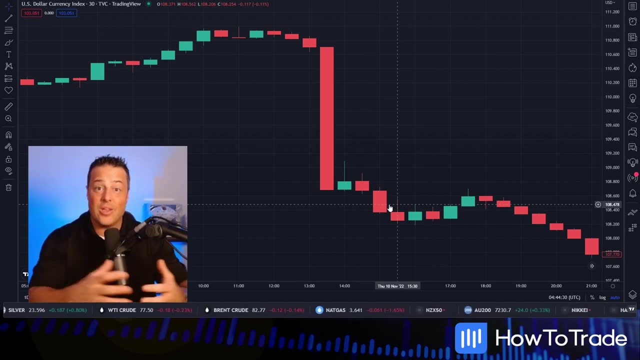 orders hits the market, there's your bearish directional move, Number three. well, in number three, and then number four. you don't get the retracement. You don't get the Wall Street rebound. Now, a lot of that has to do with this being a dollar and not a risk asset like a US 30.. But 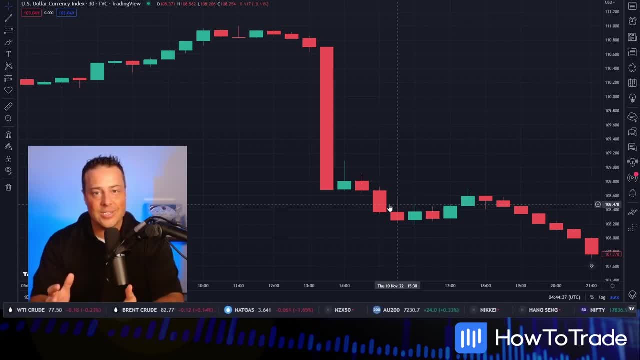 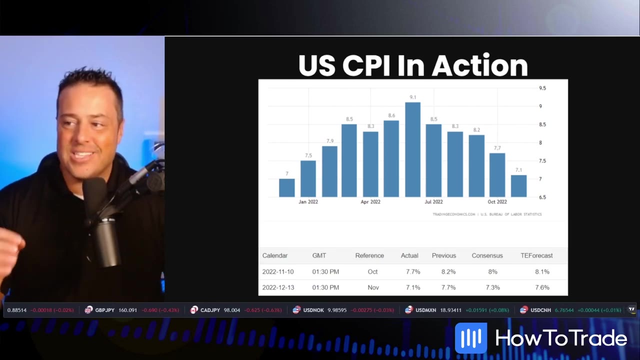 still, just because sometimes we get that big correction doesn't mean that we're going to get it every single time. So now let's look at a few keys on how to trade CPI successfully. No matter if CPI is at all time highs or if it's on a downward trajectory, there's a few things. 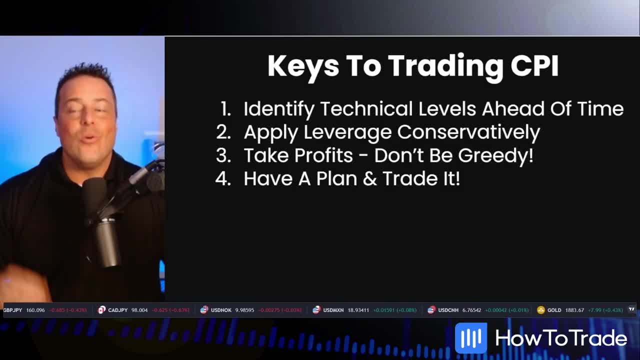 that we need to do to trade it effectively. Number one: we have to identify our technical levels ahead of time. Understand that when that CPI number drops, price action is going to be violent, It's going to be unpredictable, It's going to be all over the charts. Have your technical.